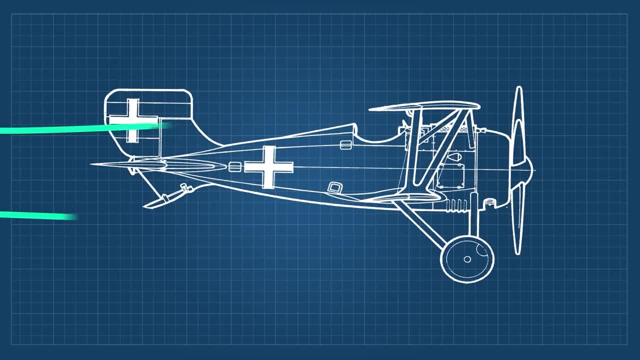 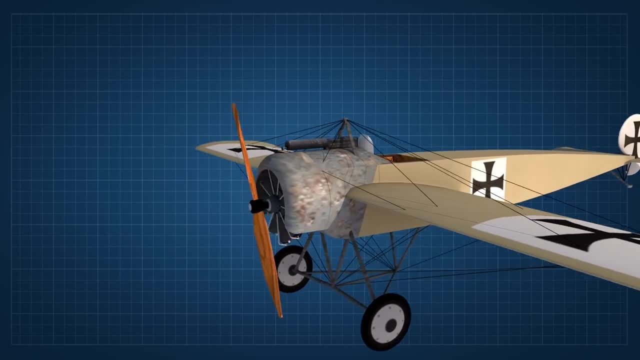 an extra cooling system, since it will be cooled by the air. But this arrangement will produce a lot of air drag, slowing the plane down during its flight. Many early airplanes use this kind of engines to simplify the cooling problem. The other kind of arrangements especially. 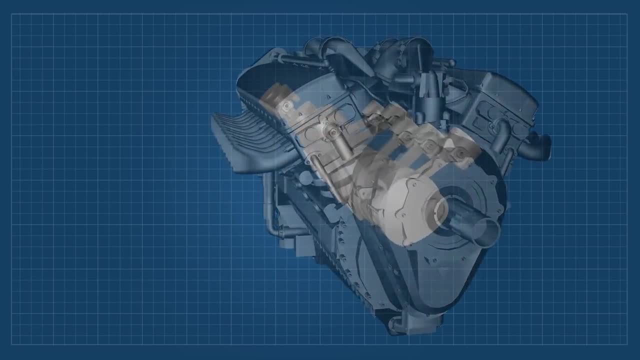 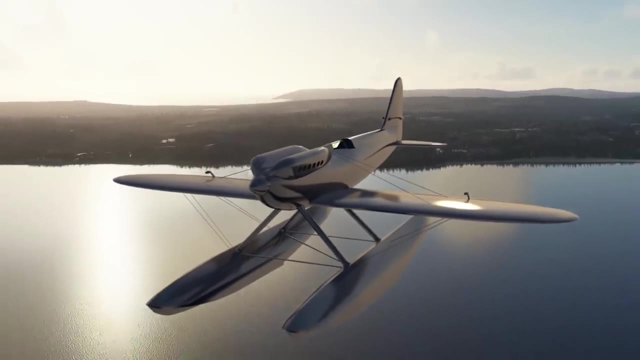 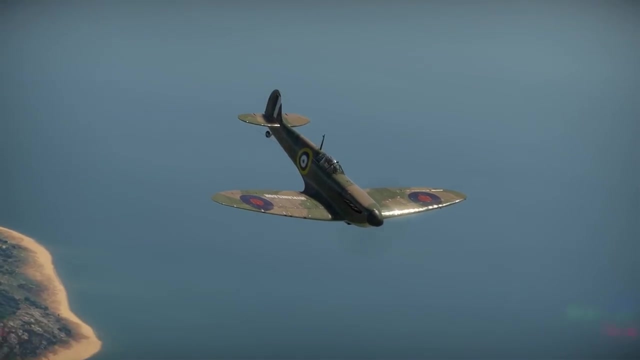 the V-type will allow for a slimmer design and better aerodynamics, But the cooling will be more critical, relying on more complex cooling systems. It's totally worth it. if you want to get the maximum speed out of the engine To go faster, a piston engine won't. do You need a better technology For that? we can. 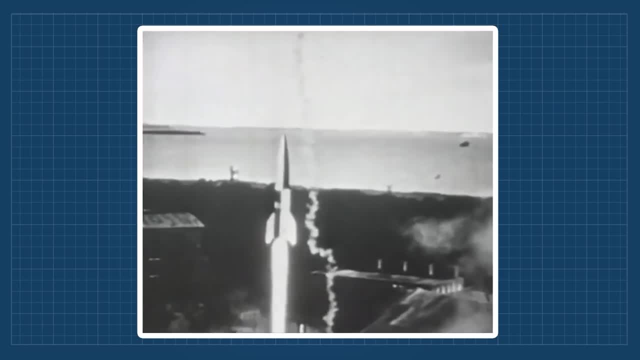 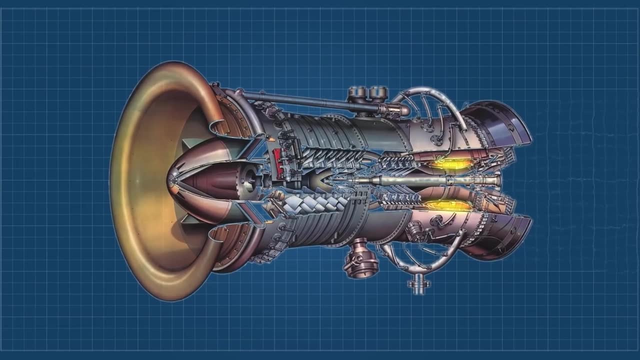 use rocket engines, But they are very inefficient and they burn fuel very quickly. Jet engines or turbines came along and they were the answer to the speed and power problem. After many years of development, they were ready to be deployed, first being used in. 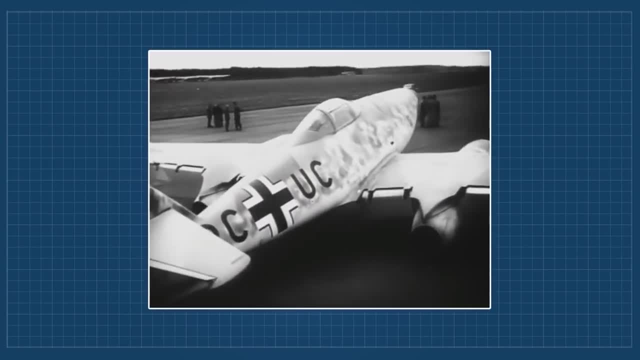 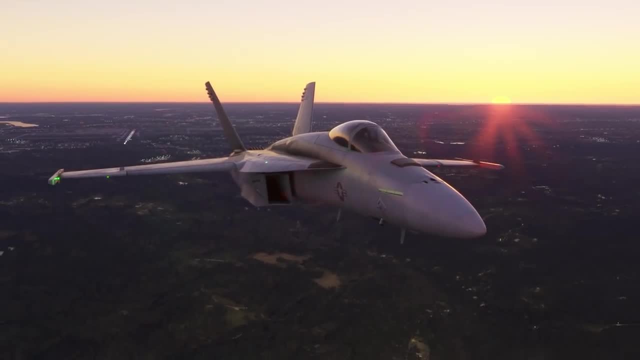 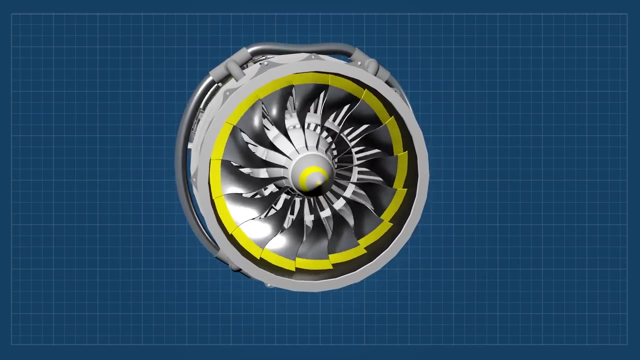 the Second World War. After a long time of development, the technology kept improving to the point it was very efficient, reliable and perfect for its use in many variants of engine types and aircraft. The turbine uses a lot of small blades rotating at high speed. The engine takes air from one. 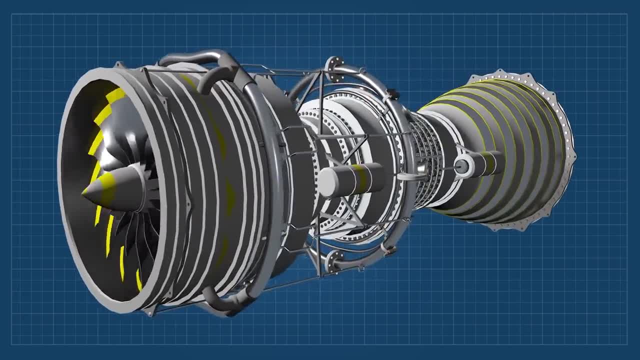 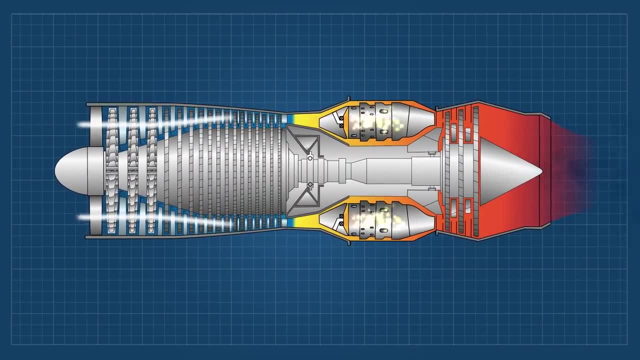 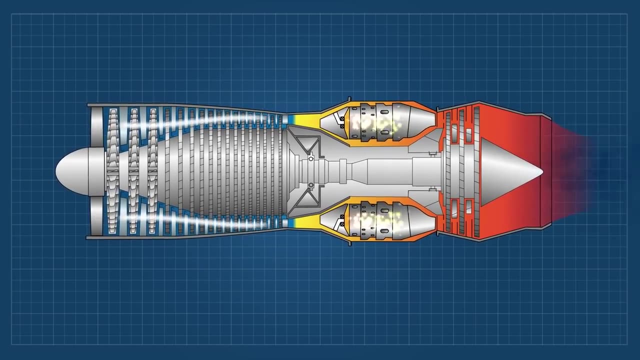 end and forces it through the different stages where it is compressed, then mixed with atomized fuel, then ignited. then the expansion of the gases will escape towards the back, forcing the rotation of the next set of blades turbine, which at the same time turns the whole system. Notice the similarity on 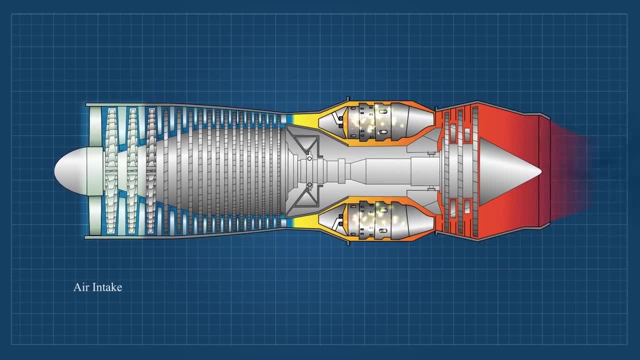 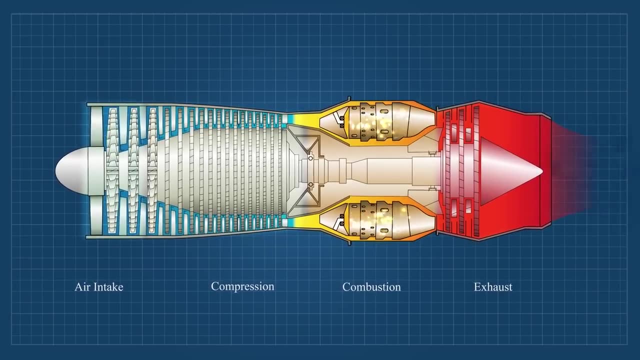 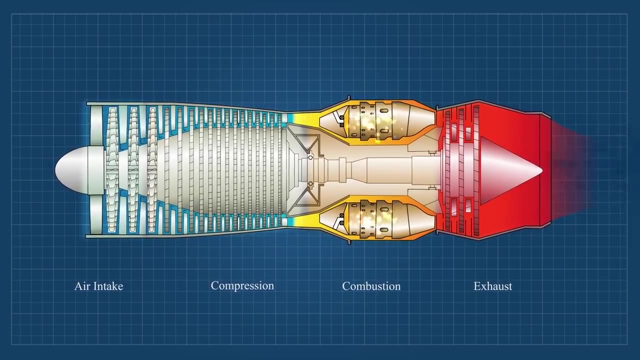 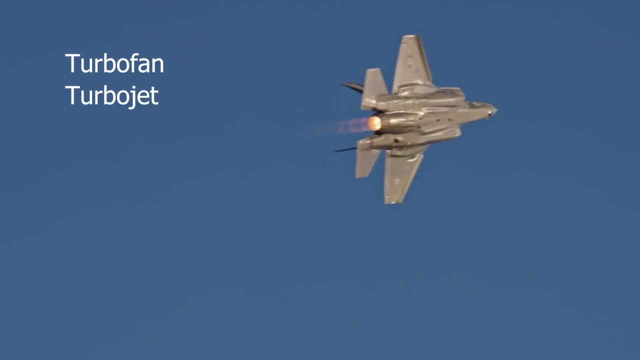 the four stroke engine cycle. in the turbojet engine we have the air intake, the compression, the combustion and the exhaust stages. but this is happening continuously, not like a cylinder, where every stage is defined by the stroke of the piston and then the explosion is the combustion. nowadays there are many type of jet engines. there are turbofan, turbojet. 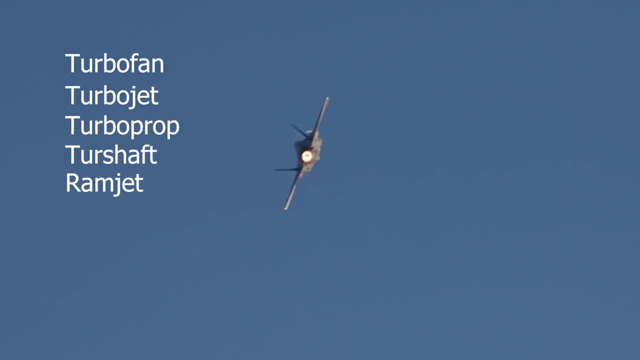 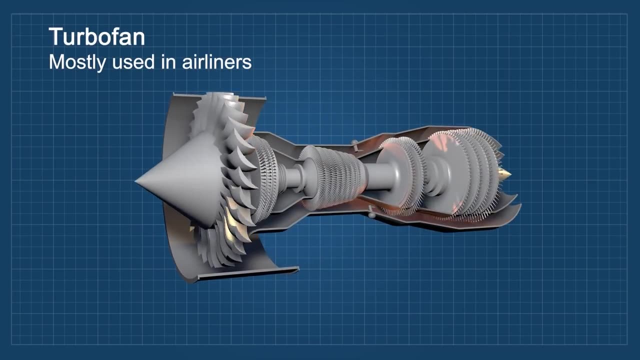 turboprop, turboshaft and ramjet engines. the most used in civil aviation is a turbofan engine. in this type of engine, there is a large fan at the front that sucks all the air in, most of which is used to generate thrust, and only a small. 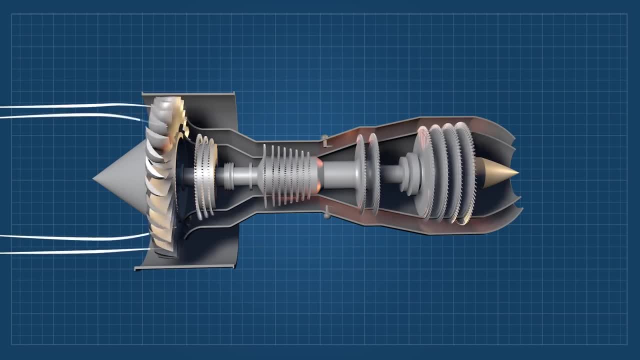 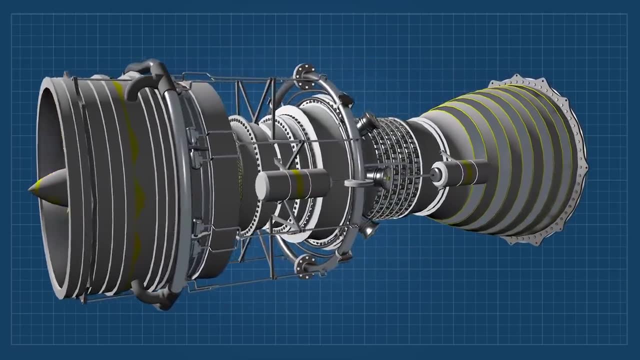 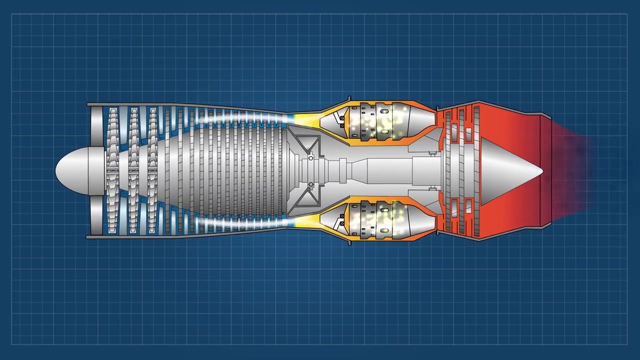 percentage actually goes into the combustion stage. the advantage of this kind of engine is that is a lot quieter and more efficient than the turbojet engines for subsonic speeds. the turbojet engine is the one that we saw in the first example, and all the air that gets in is used for the combustion process. it's 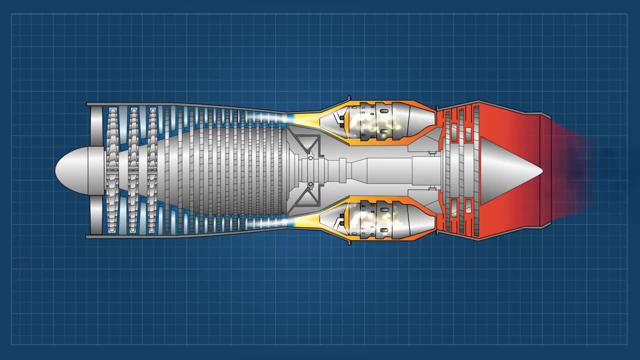 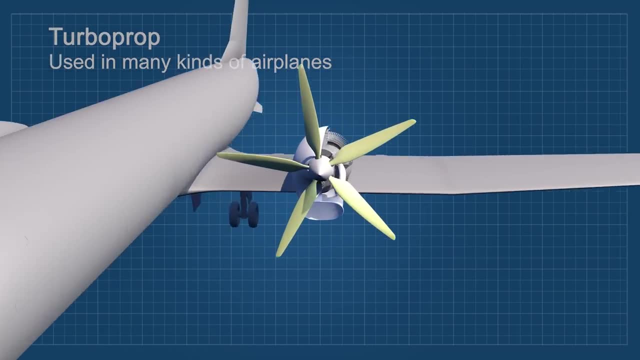 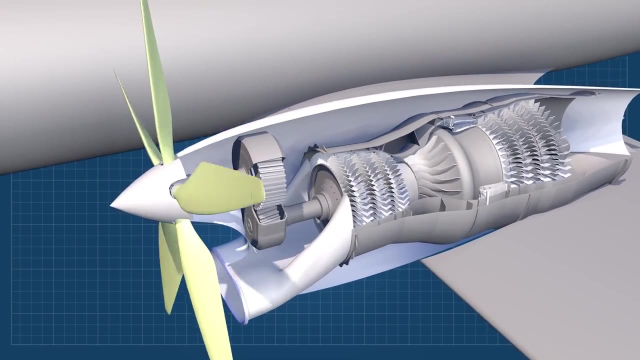 very powerful, very noisy but somewhat smaller than the turbofan engine. the turboprop engine uses the power from the turbine and through a gearbox, the rotation is transmitted to the propeller. compared to turbofans, turboprops are most efficient at flight speeds below 725. 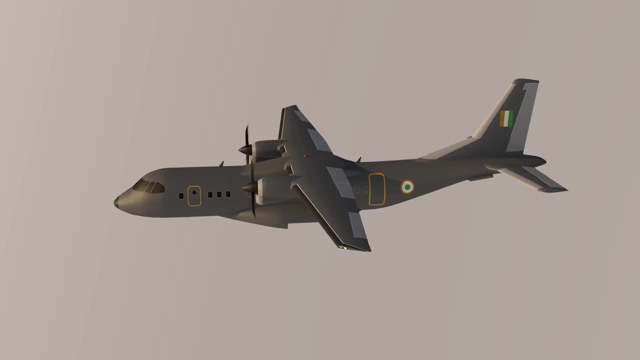 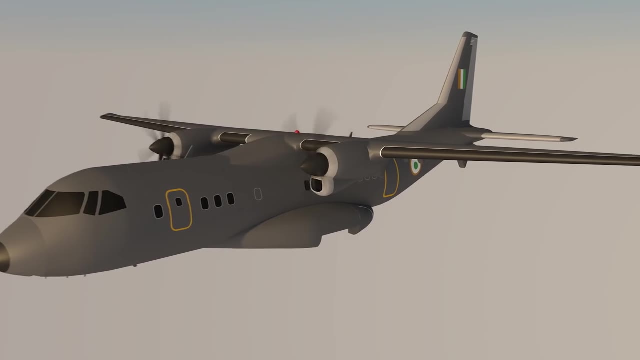 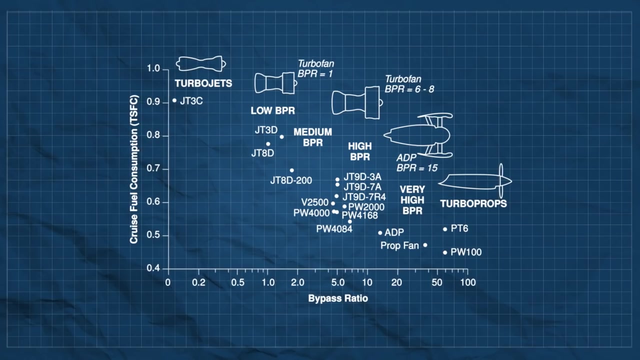 kilometers per hour or 450 miles per hour, because the jet velocity of the propeller and the exhaust is relatively low. modern turboprop airliners operate at nearly the same speed as small regional jet airliners, but burn 33% less fuel per passenger, however, compared to a turbojet which can fly at high altitude for 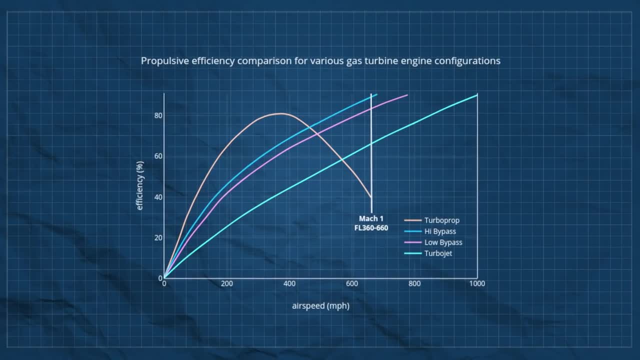 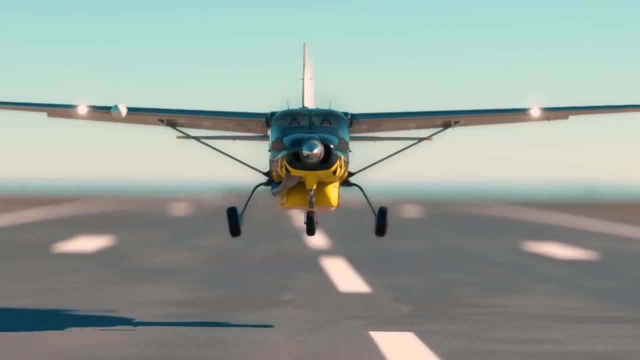 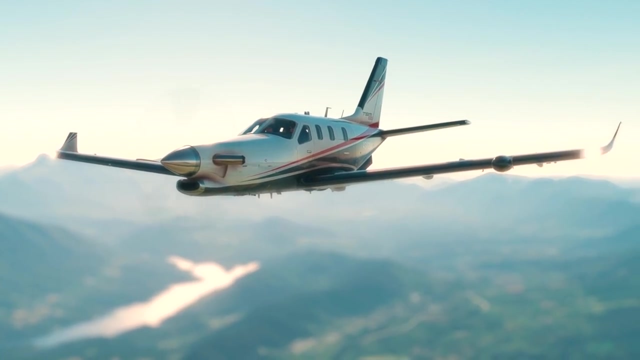 enhanced speed and fuel efficiency. a propeller aircraft has a lower ceiling and, compared to piston engines, their greater power to work and their power to weight ratio, which allows for shorter takeoffs and reliability, can offset their higher initial cost, maintenance and fuel consumption, also as jet fuel. 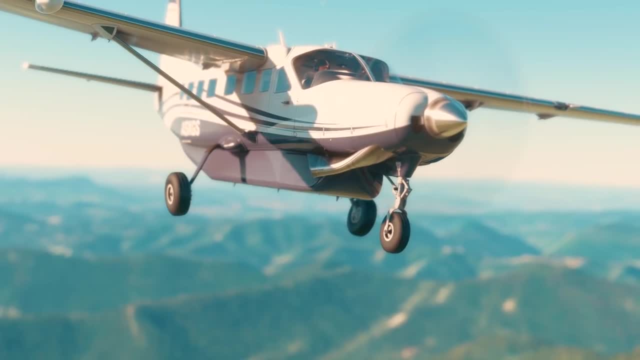 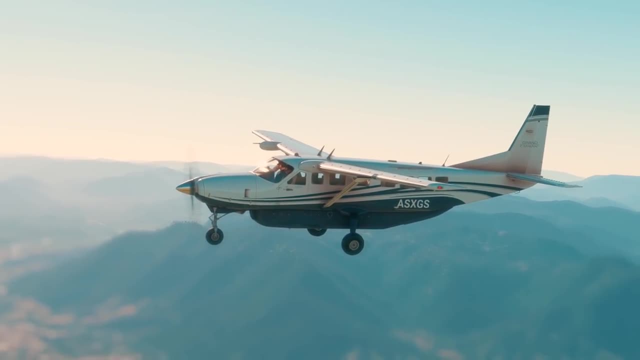 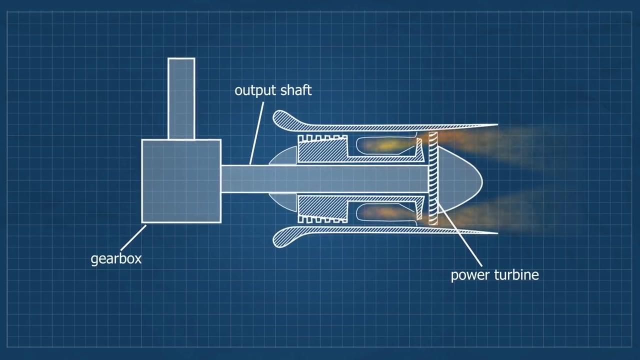 can be easier to obtain than aviation gasoline in remote areas. turboprop powered aircraft like the Cessna Caravan and Quest Kodiak are used as bush planes. the turboshaft engine is similar to the turboprop, but it is connected to a big shaft and it's normally used for helicopters. the workings of 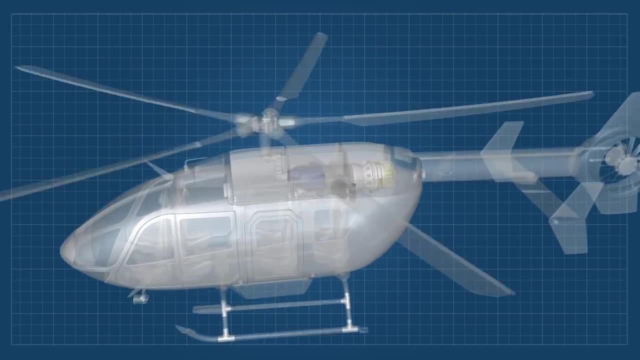 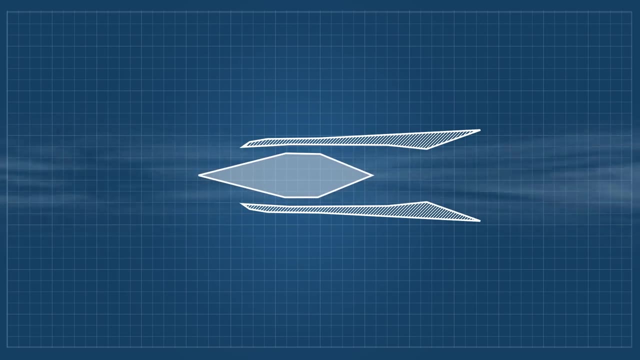 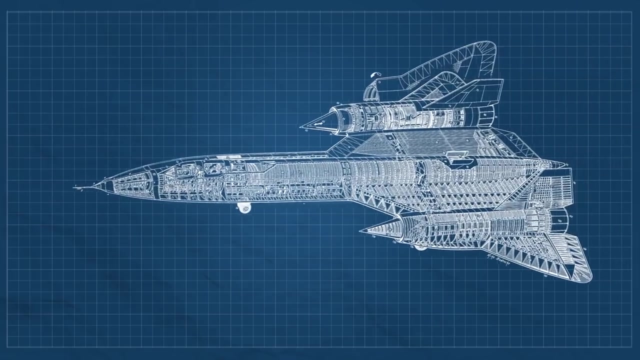 the whole system is practically the same. it can also be used for military tanks and even boats. lastly, we have the ramjet engines. these engines are more like a rocket, with the difference that they can only produce thrust once they have a fast airflow to start working. in other words, the airplanes have to be 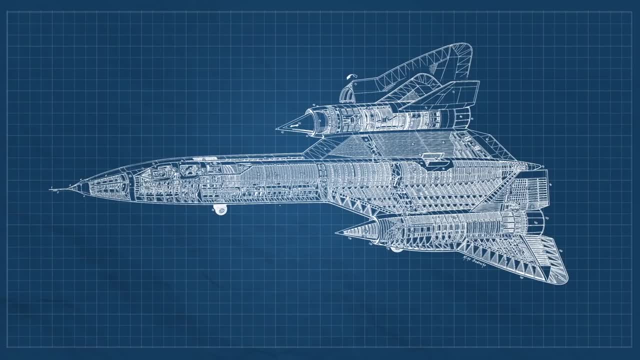 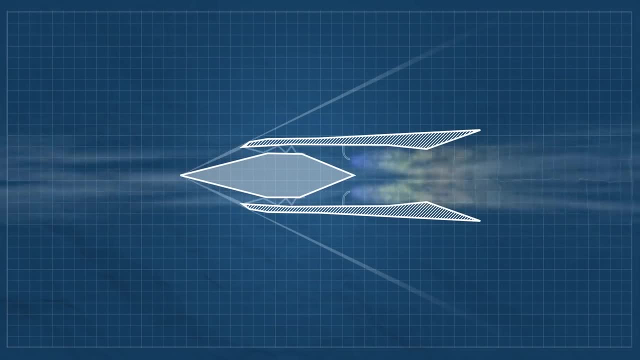 flying already at a fast speed. for this engine to work, this engine does not have a set of blades like the turbines. it has very few moving parts and it relies on its shape to slow down the supersonic airflow at the intake to a subsonic speed, driving the air to a compression stage and then burning the fuel with. 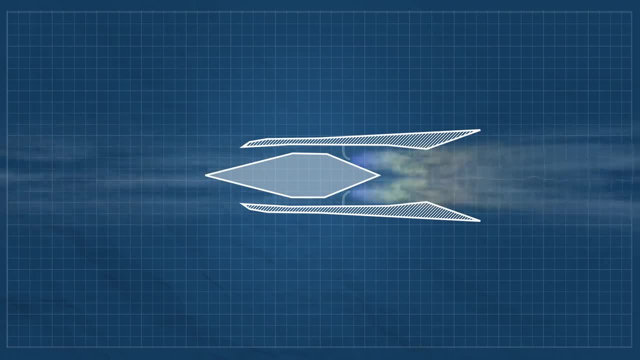 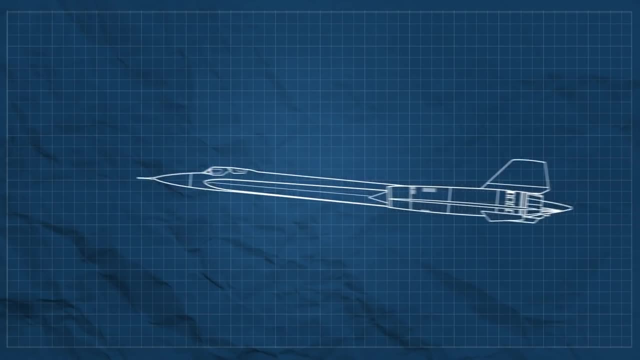 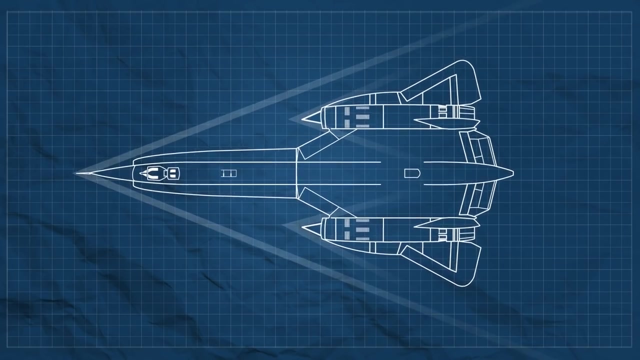 this compressed air to generate supersonic thrust towards the nozzle. this engine is used in the SR 71 Blackbird. although you might wonder then, how can this airplane take off if the ramjet engine can only work at a supersonic speed? well, this airplane has a turbojet engine nested inside the ramjet. 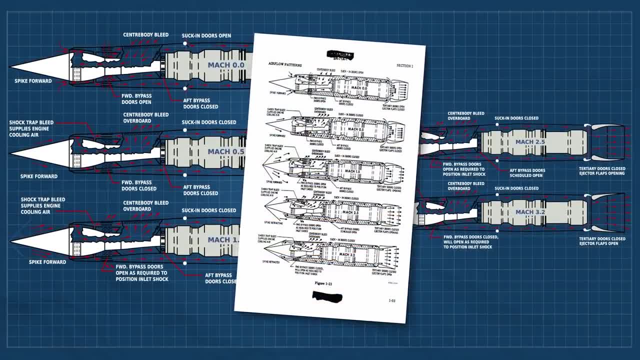 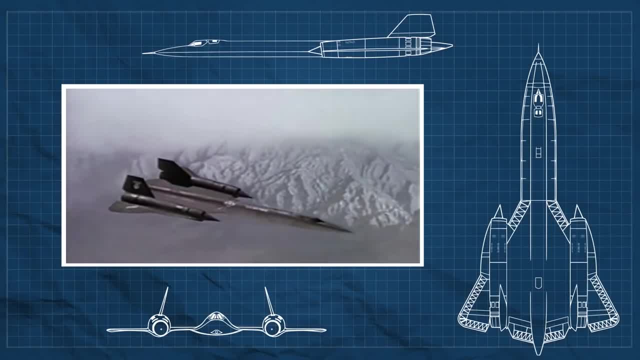 it's a two-in-one solution. once the plane reaches the speed needed, then there is a bypass that will allow the engine to work mostly as a ramjet engine. it's a bit more complicated than that, so I suggest you watch the videos from other YouTube channels, which links I provided in the description below, to have a more. 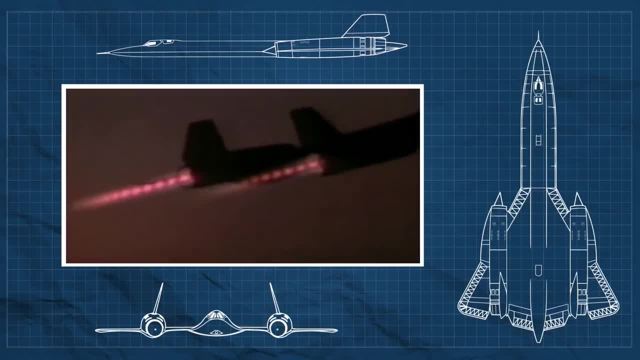 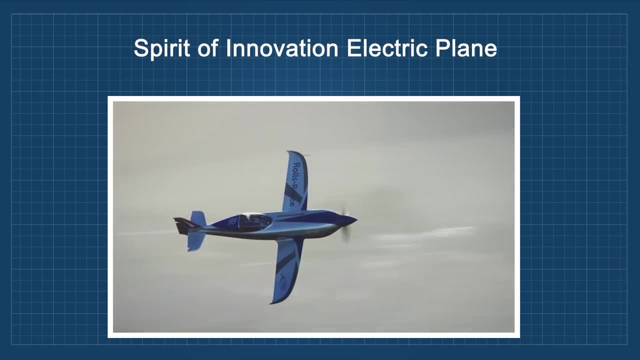 detail and better understanding on how the engine works on the SR 71 Blackbird. I could keep talking about other types of propulsion systems for aircraft, like the new electric motors, in which the only limitation is that the engine can only work at a supersonic speed. we have now is the amount of energy we can store in our current battery. 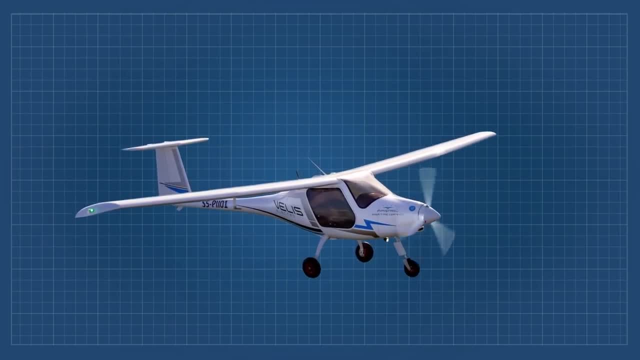 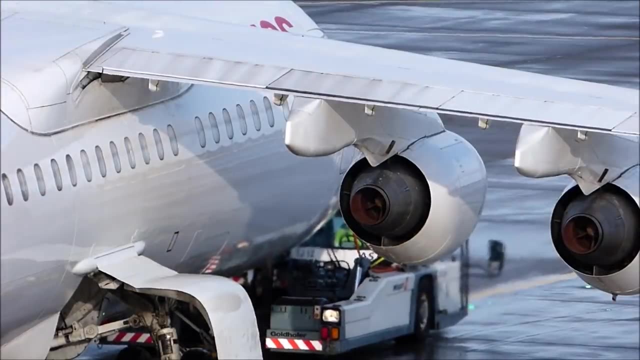 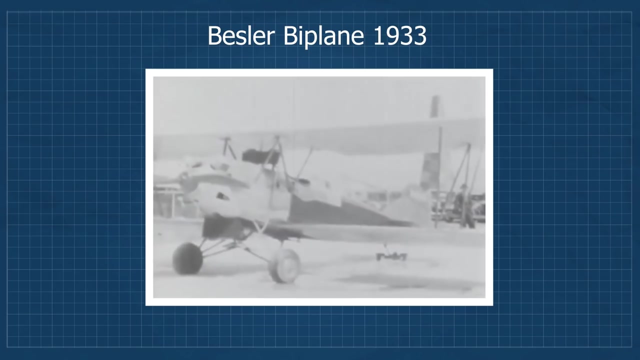 technology, but it promises a great future for electric aviation. but I think this deserves an entire video on its own. I will only mention a few weird propulsion systems that are not practical or not developed enough to be used in aircraft. going back in time, we have a steam propelled aircraft, one of 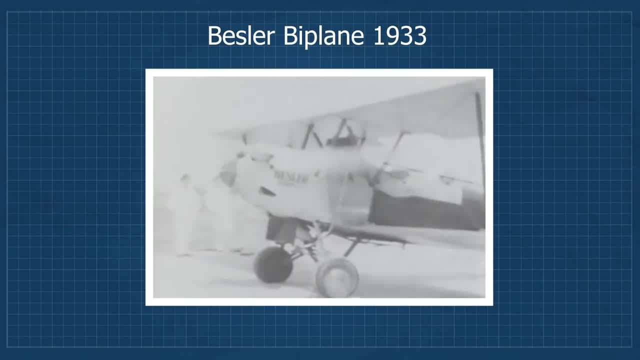 the most successful was the Bessler biplane, but this steam engine was heavier, less efficient and more complex than I thought it would be. but I think it's worth mentioning that the Bessler biplane is the most efficient and the most efficient of the Bessler biplanes, but this steam engine was heavier, less efficient and more complex than a. 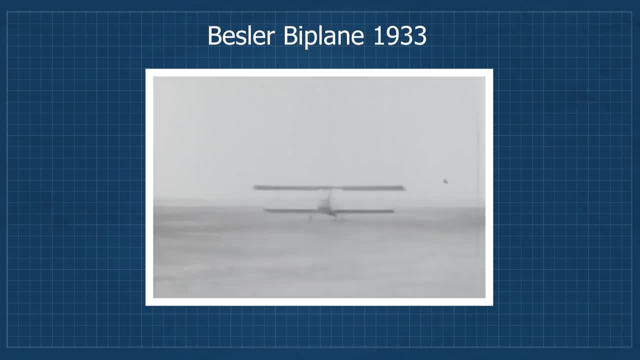 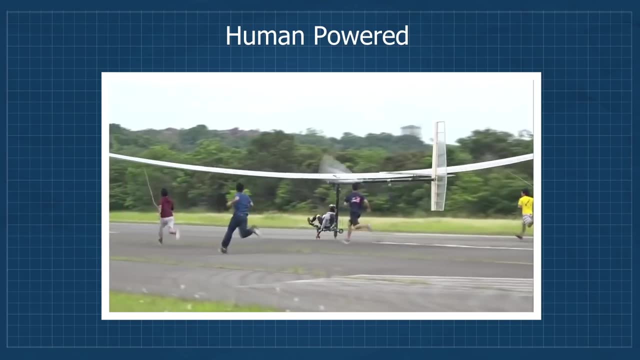 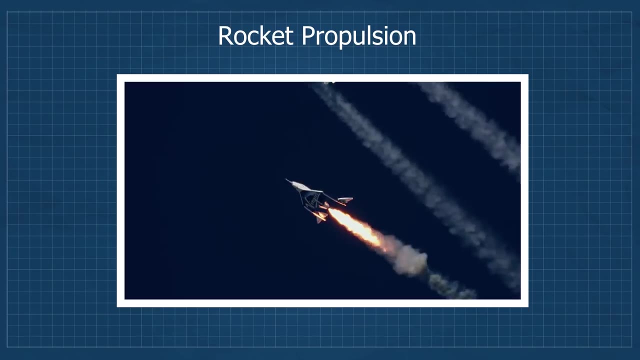 conventional internal combustion engine. it could not compete with the combustion engines so it was never put into production. human-powered aircraft is another peculiar type of propulsion. but it's completely possible only in good weather conditions and if the person is not hired, then we have rocket propulsion to go at the fastest speed possible, but for a brief moment and the 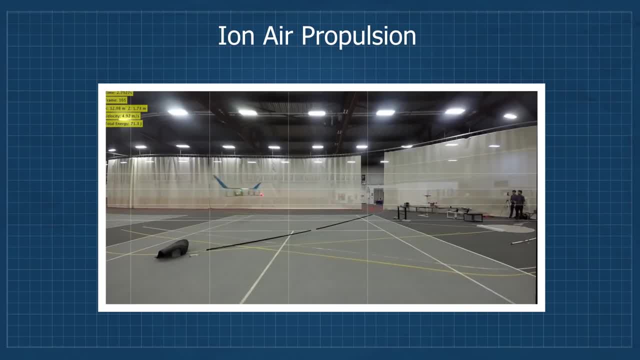 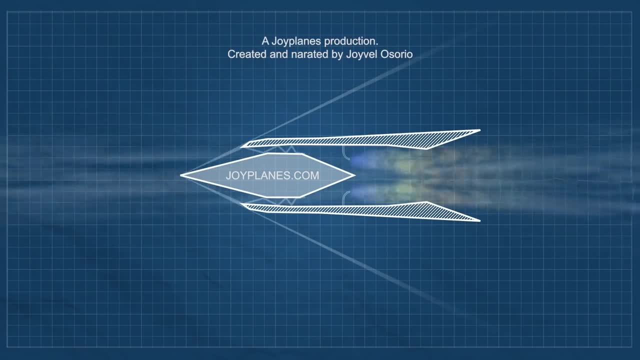 final one I'm going to mention is the ion propulsion, a very new technology, and that's it for this video. if there's another type of engine you would have liked me to mention, just leave it in the comments below, and I hope you enjoyed this video. thanks for watching and I'll see you. next time.